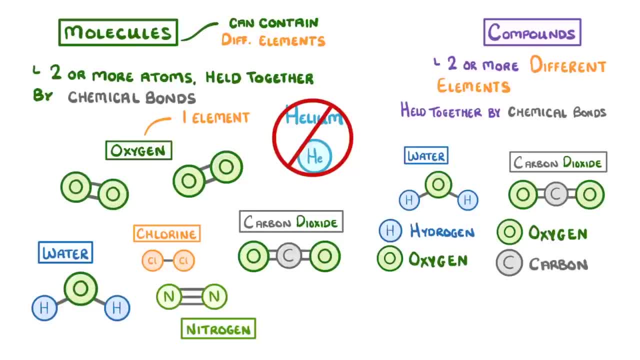 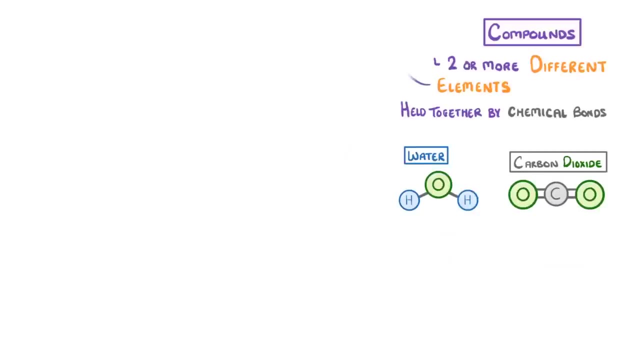 because it contains the elements oxygen and carbon. However, molecules like oxygen, chlorine and nitrogen aren't compounds because they only contain one type of element. Another key feature of compounds is that the elements involved are always found in the same proportion. So if we take a look at our molecules, we'll see that they contain two or more elements. 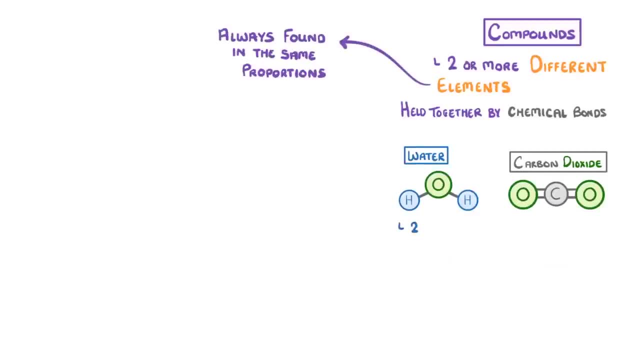 For example, water always has two hydrogen atoms and one oxygen atom. This allows us to write formulas for them using their chemical symbols and the numbers of each atom. So the formula for water would be H2O, with the two written in subscript, which means: 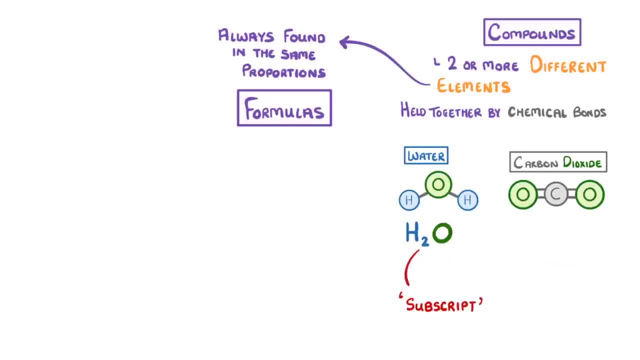 it's smaller and slightly lower down, and this signifies that there are two hydrogens in the molecule, Whereas if there was only one atom of that element, like with oxygen, then we wouldn't write any number in subscript. So carbon dioxide is CO2, because there are two oxygen atoms but only one carbon atom. 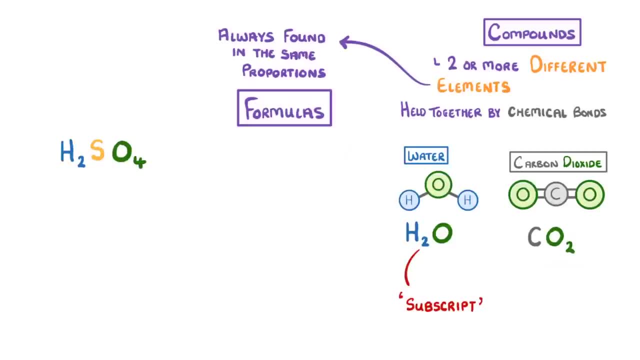 A more complicated example is H2SO4.. And if you're ever not sure what any of the symbols mean, remember, you can just look them up on the periodic table, because it will also have their full name. If we read it letter by letter, we can see that carbon dioxide is equal to CO2.. 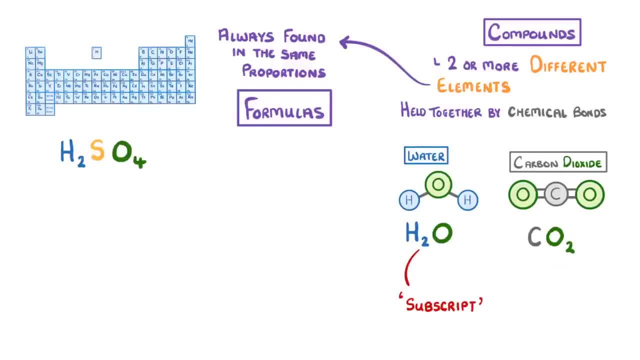 So if we write it letter by letter, we can see that each molecule of sulfuric acid contains two hydrogen atoms, one sulphur and four oxygens, Although you wouldn't be expected to know that they fit together like this, we're just doing it to show you how it works. 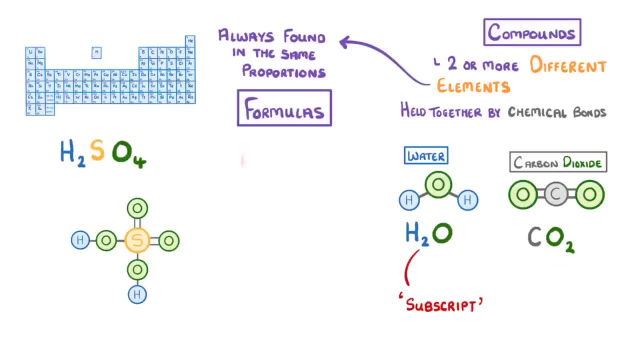 Sometimes you might also see brackets in formulas, such as in calcium hydroxide. Just like in maths, the brackets effectively group together everything inside them and then the number on the outside of the brackets. So that's the first one. The second one tells us how many of those groups there'll be. 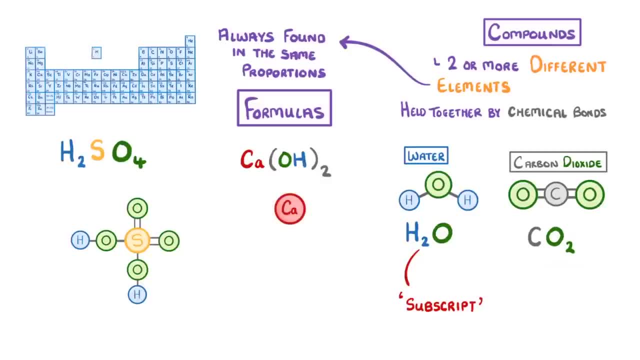 So in this case, there's one calcium atom and two groups of OH. The compounds we've seen so far have all been relatively small, containing just a few atoms. Some compounds, though, can contain millions or billions of atoms. For example, common table salt is actually a compound called sodium chloride, which has 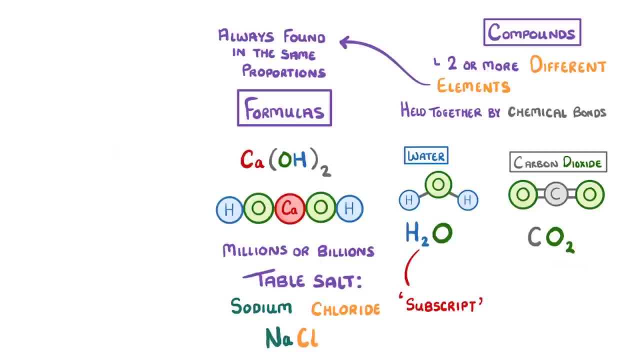 the formula NaCl. From the formula you might have noticed that sodium chloride contains a lot of sodium. In particular, you might think that it represents little molecules made of one sodium and one chlorine, But sodium chloride actually exists as huge structures containing millions or billions. 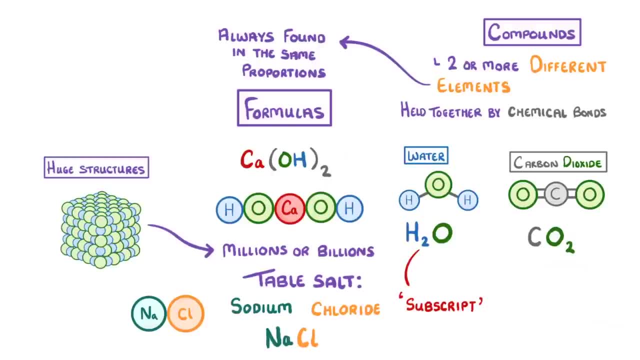 of atoms. We covered the details in another video, but you can generally tell which compounds will form large substances rather than molecules. because the bonds between the atoms are ionic bonds And because they form such large substances they don't count as molecules. 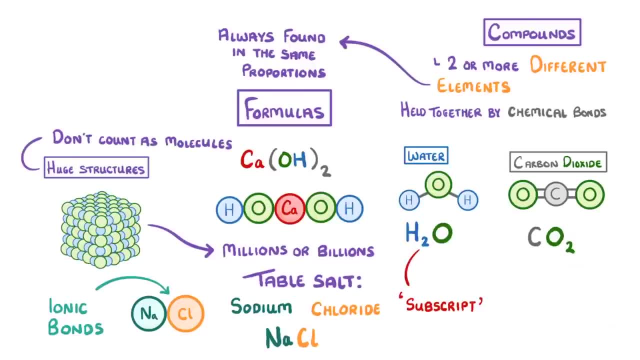 The first one is called sodium chloride, The second one is called NaCl, The third one is called NaCl. The formula for these non-molecular compounds, though, is still important. It just acts as more of a ratio, For example, with sodium chloride. we can see that sodium and chloride are in a one-to-one. 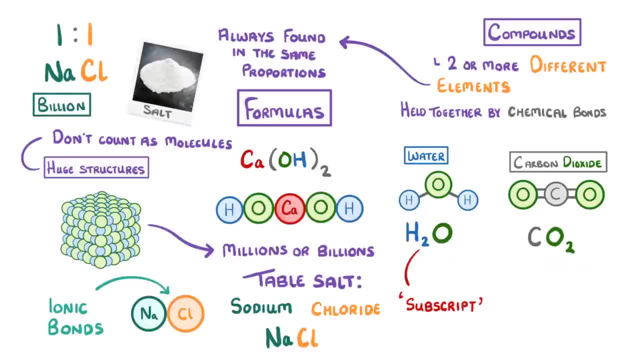 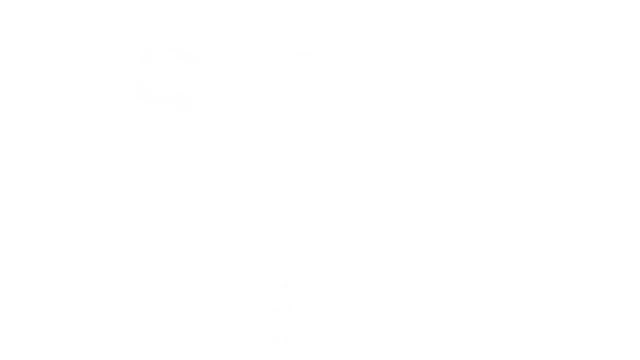 ratio. So if a crystal of salt contained one billion sodium ions, it would also contain one billion chloride ions. Before we finish, I just wanted to quickly mention mixtures which consist of two or more substances. They are not chemical compounds. 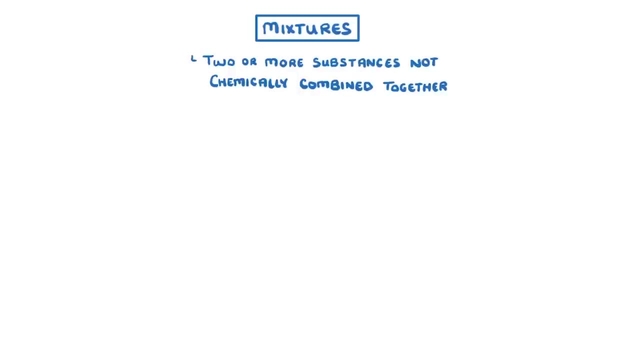 They are not chemical compounds, They are just physically combined together. So if we took a beaker and we put in some oxygen molecules, some sodium chloride, which is a compound, some individual helium atoms and a molecule of carbon dioxide, this entire. 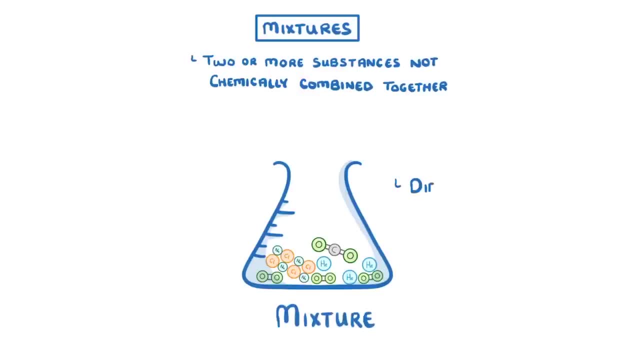 thing would be a mixture, because it contains lots of different substances, but, importantly, they haven't reacted with each other, So there's no chemical bonds between the individual substances. They've just been physically combined. That's it mixed together And because of this we can easily separate them using physical methods. 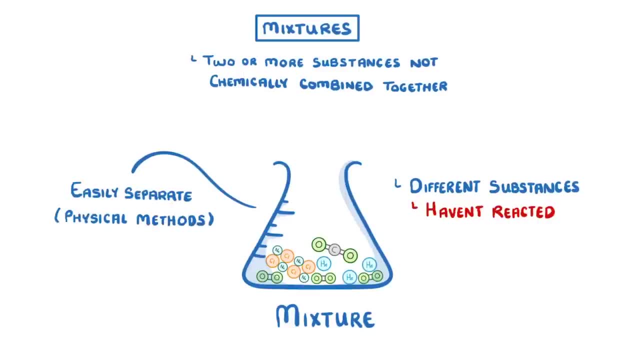 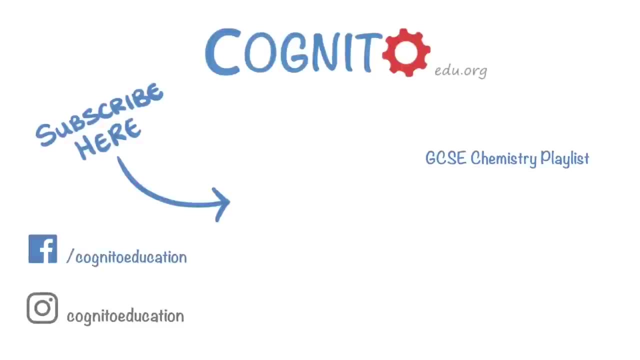 like filtration, crystallization or distillation, which we cover in other videos. Anyway, that's all for this video, So we hope you enjoyed it. If you did, please give us a like and subscribe and we'll see you next time.